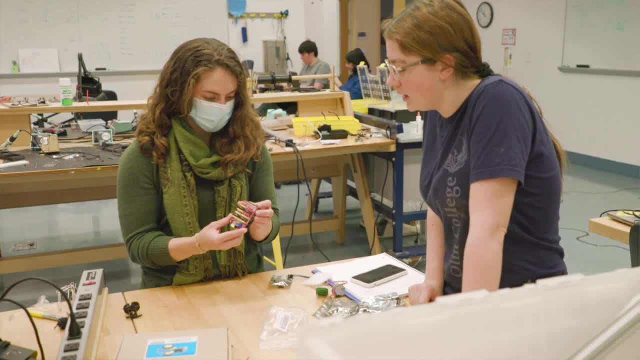 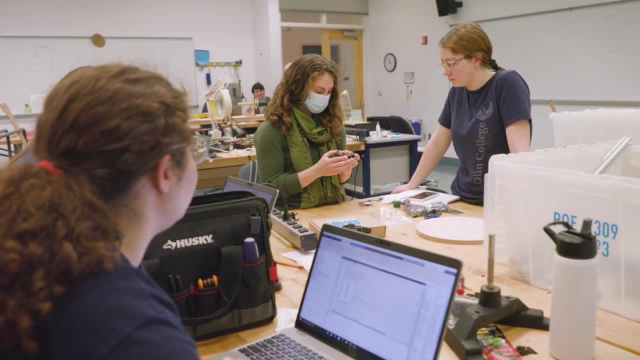 The students start with three mini-projects. So sort of the basics of how do you work with an Arduino, how do you work with a microcontroller, how do you work with different actuators and sensors. So we're building up their skill sets. 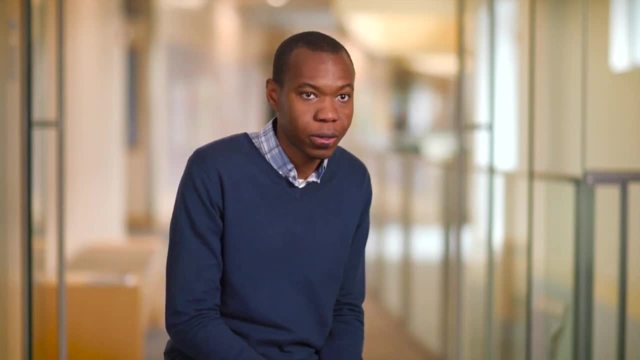 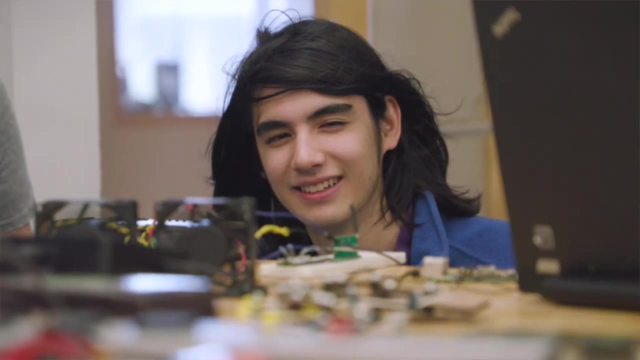 We want students to practice working in teams, And this is crucial to how engineers work in the real world. Engineers don't work in isolation, they work in teams, And so we try to use the Pi project, the Pi class, as an opportunity to help students build that competency. 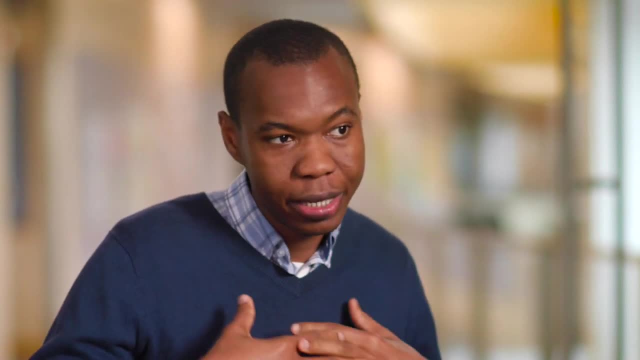 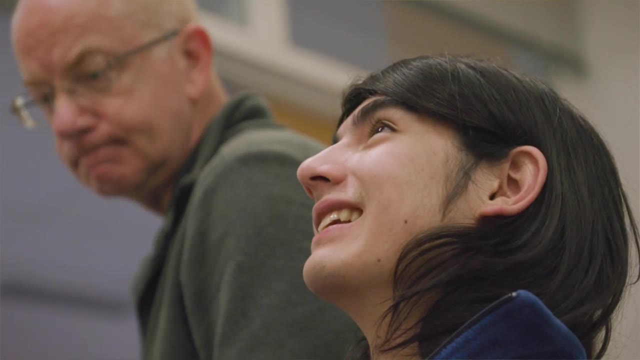 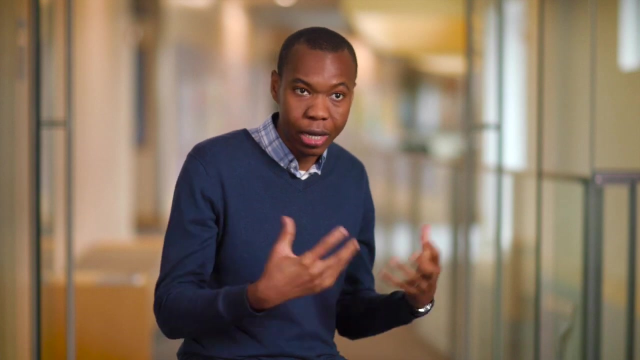 As a teaching team, we do not stand in front of the class disseminating information to students, but we actually work alongside them And that helps them to learn more concretely and more deeply about things. It allows them so many varied opportunities to ask questions about how their learning. 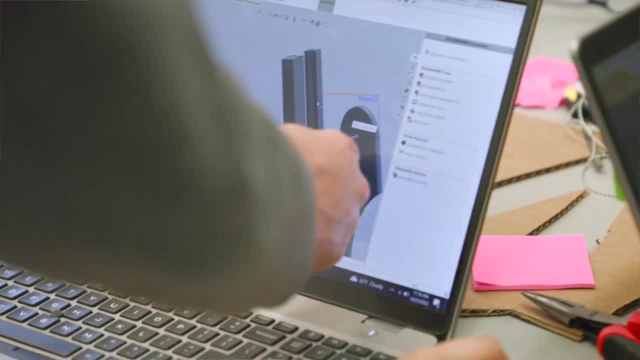 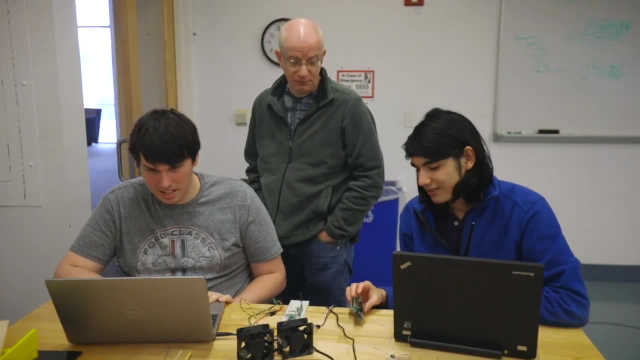 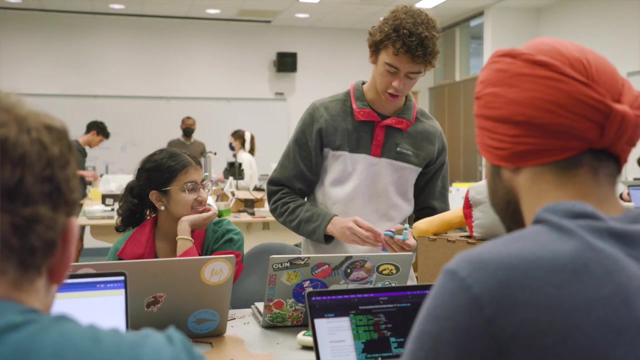 is going. It's also taught explicitly in a multidisciplinary team of faculty, And so we have people from mechanical engineering, robotics, computing, electrical engineering that make up a diverse teaching team, And so students have people with expertise in all the relevant disciplines. 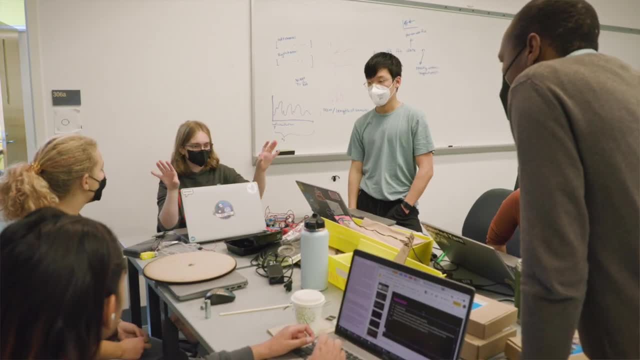 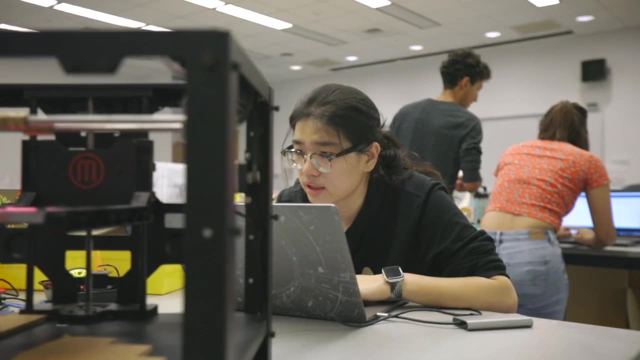 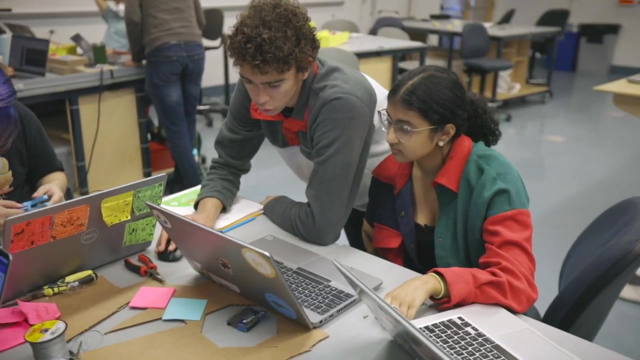 as resources for them. In the final project. students have about six, seven weeks to do some integrated project, Whatever they are passionate about and excited about. each team has a budget that we give them some money to spend, And then we're there to sort of guide them through this process. 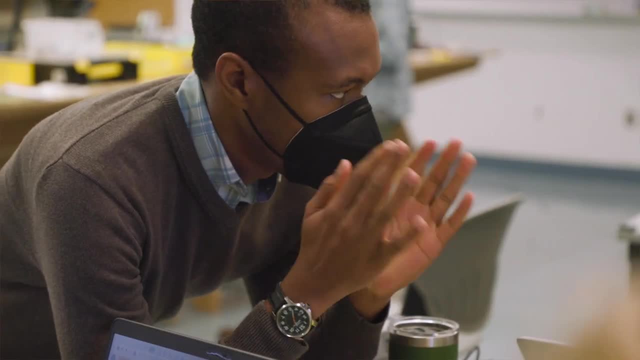 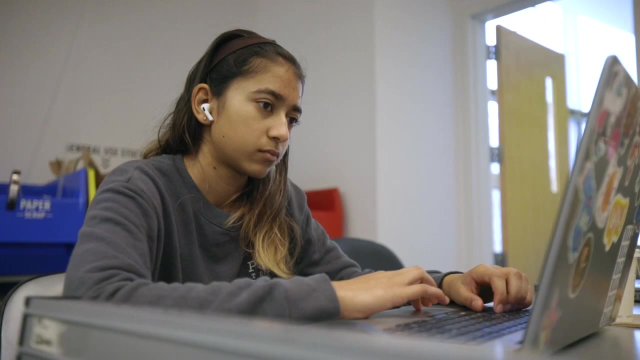 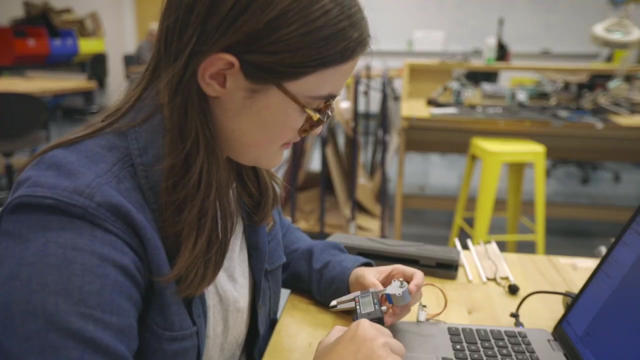 I think Pi is a very crucial part of the Olin curriculum in that it provides students with a second year experience on how to design real things. It's mostly taken by sophomores. It gives students, before they declare their major, an opportunity to sort of sample different. 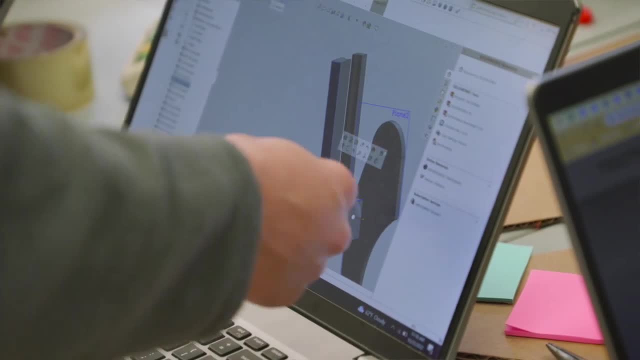 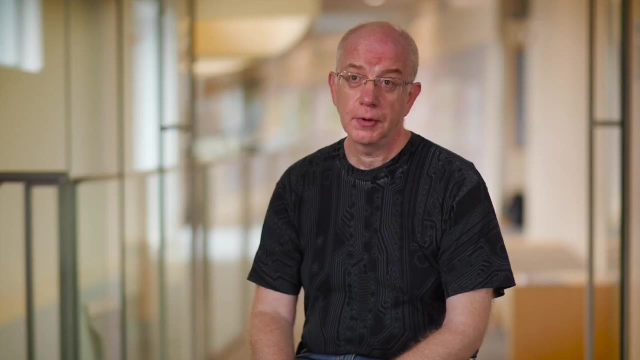 mechanical engineering, electrical engineering, computing, robotics, And so the fact that this is coming kind of so early in the curriculum, I think, is kind of a thing that makes it a signature Olin experience, So like it doesn't read until we pass the A-levels, right. 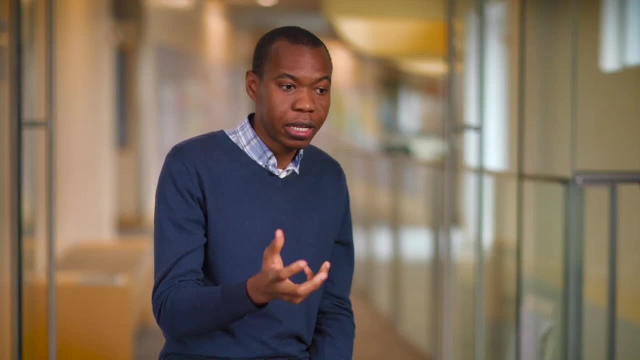 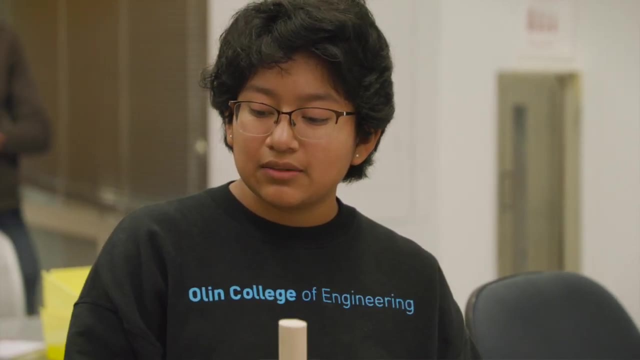 It gives them confidence to know that they can ideate and design, analyze and construct things that have real value. Olin students are really committed to trying to make a difference in our lives as students. at the same time, they're really good about talking to their teammates and being honest, and